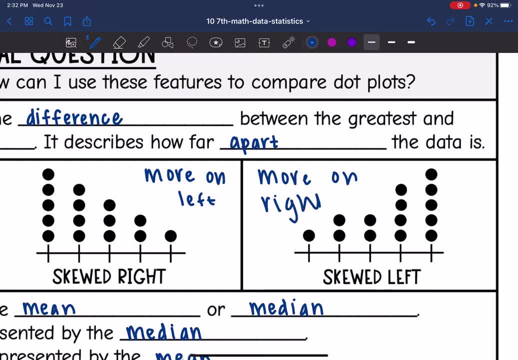 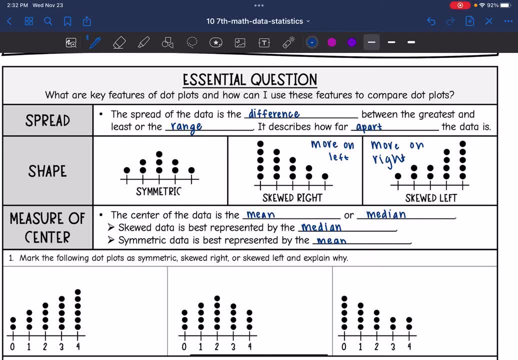 means skewed left. So let's talk about how to best determine the measure of center of dot plots. So the center of data is either going to be the mean or the median. Skewed data like this is best represented by the median or the middle. And then symmetric data is best represented by the mean or the. 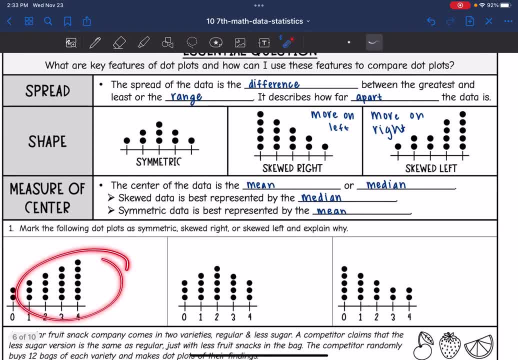 average. So let's look at these right here and we're going to mark them as symmetric, skewed right or skewed left. And then we're going to mark them as symmetric, skewed left or skewed and we're gonna explain why. So this one would be skewed left. 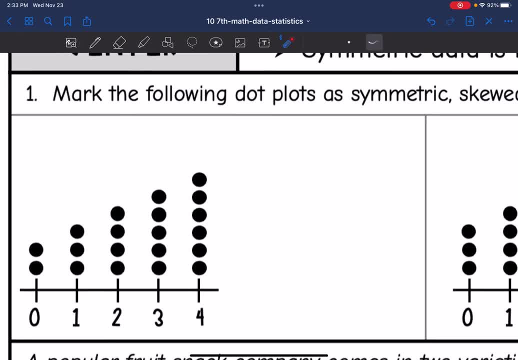 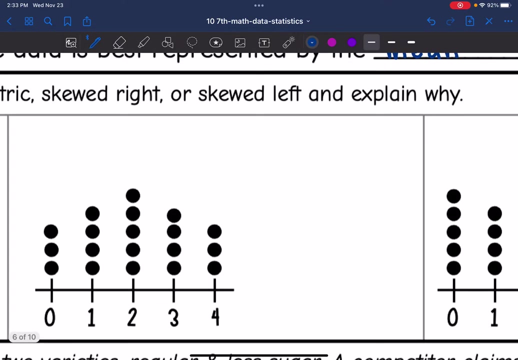 because we have more data on the right, So it is skewed left because there is more data on the right. This one right here is pretty symmetrical, It is not skewed one way or another, it is evenly spread. And then this last one: we have more data on the left. 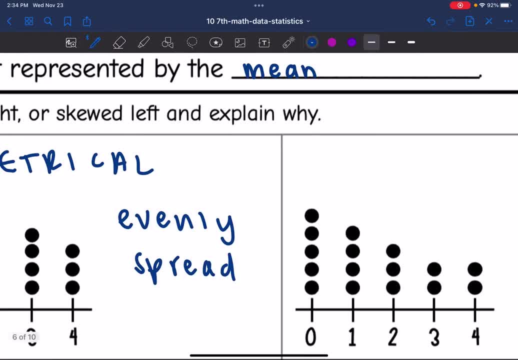 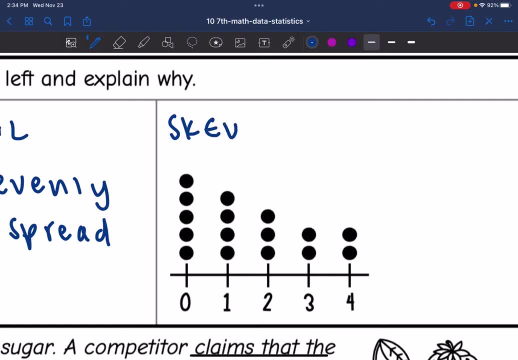 so it is skewed right. And then this last one: we have more data on the left, so it is skewed right. And then this last one: we have more data on the left, so it is skewed right. And then this last one: we have more data on the left. 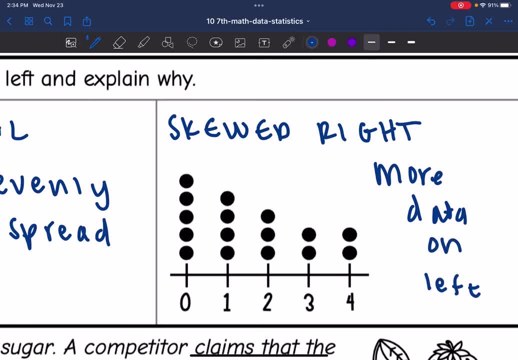 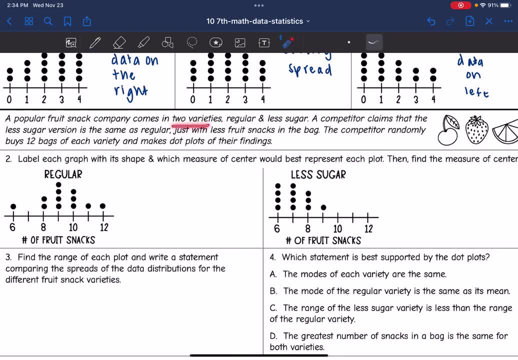 so it is skewed right, Okay. so let's look at this next scenario. It says a popular fruit snack company comes in two varieties: regular and less sugar. A competitor claims that the less sugar version is the same as the regular, just with less fruit snacks in the bag. 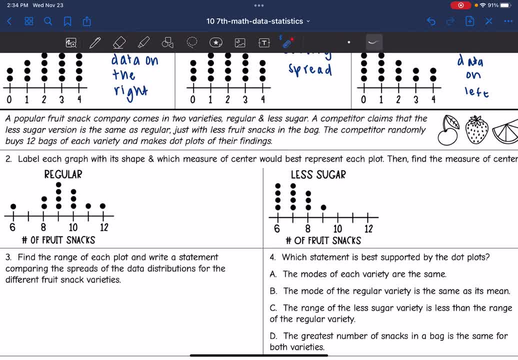 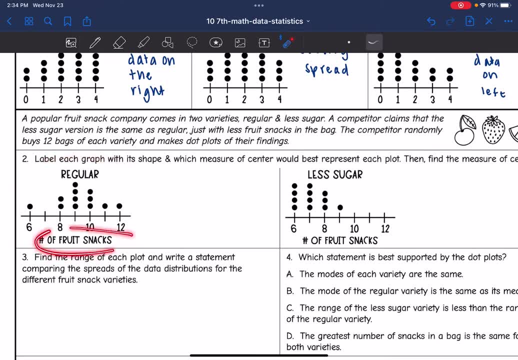 So the competitor randomly buys a bag of fruit snacks, buys 12 bags of each variety and makes a dot plot of their findings. So here is the regular and the number of fruit snacks in each bag, and then here is the less sugar and the number of. 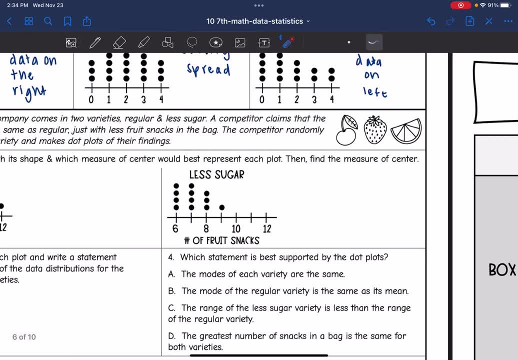 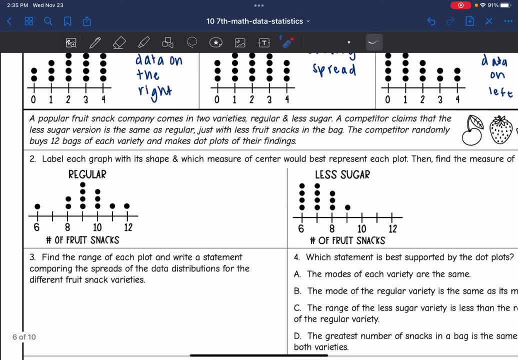 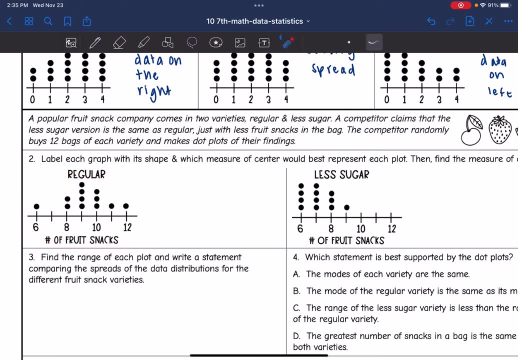 fruit snacks in each bag. So let's label each group with its shape and which measure of center would be best for each plot, and then we're actually going to find the measure of center. So this one. it is not perfectly symmetrical, but I would say that it is symmetric because 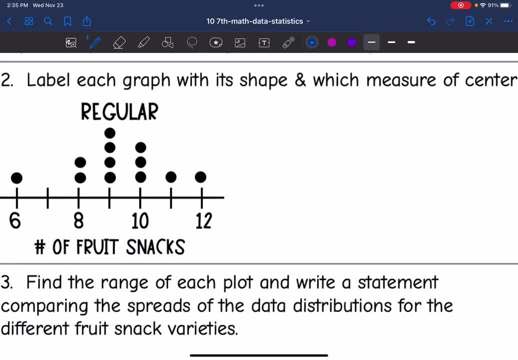 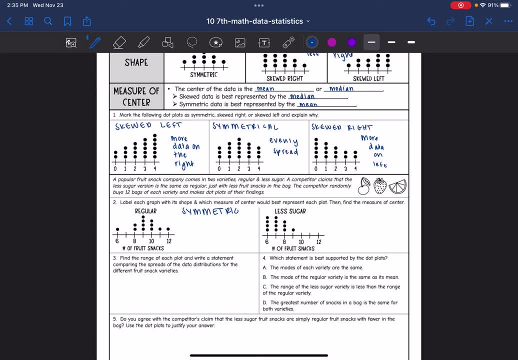 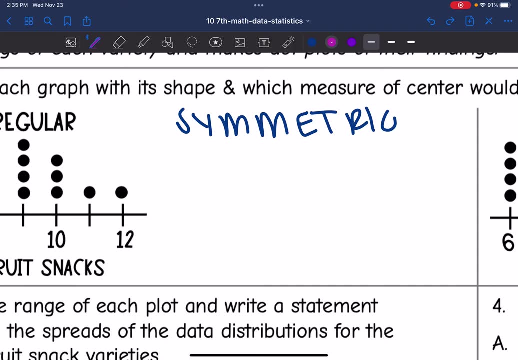 overall, it is evenly spread. So this is symmetric and symmetric, remember, that means that the mean is going to be the best measure of center. So we need to find the mean of this data set. So there are one, two, three. 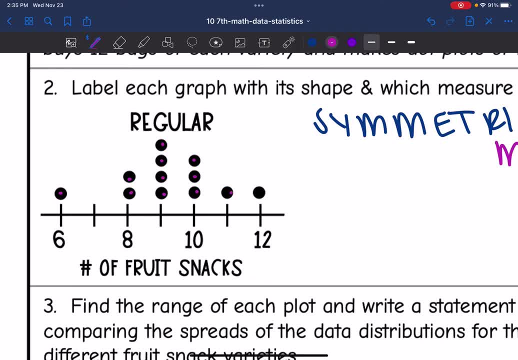 four, five, six, seven, eight, nine, ten, eleven, twelve data points, just like they told us there would be, and now I'm going to find the mean. So I would do six, there's one, six plus there's two. 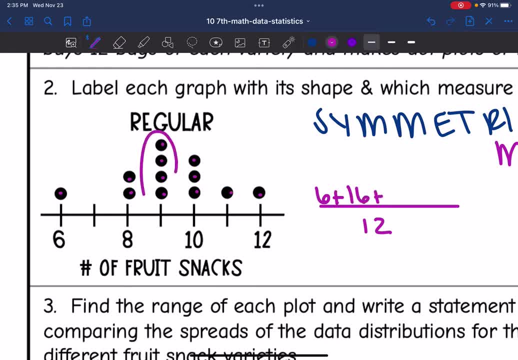 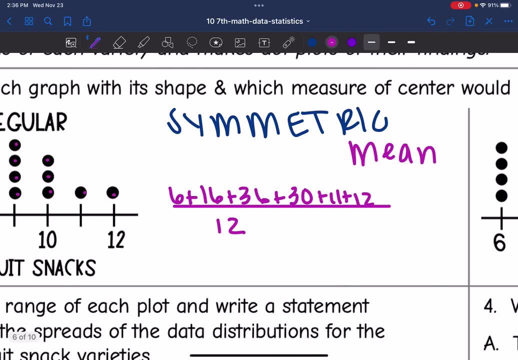 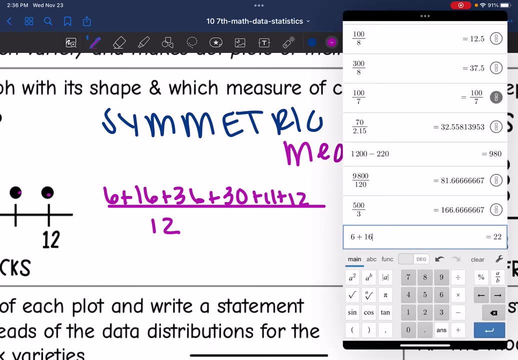 eights, so that's 16,, plus there's four nines, so that's 36, plus three tens, so 30, plus 11, plus 12.. So I need to do 6 plus 16 plus 36 plus 30 plus 11 plus 12 and then divide it by 12.. So 6 plus 16 plus 36. 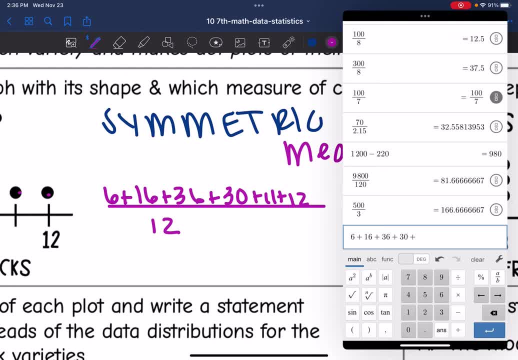 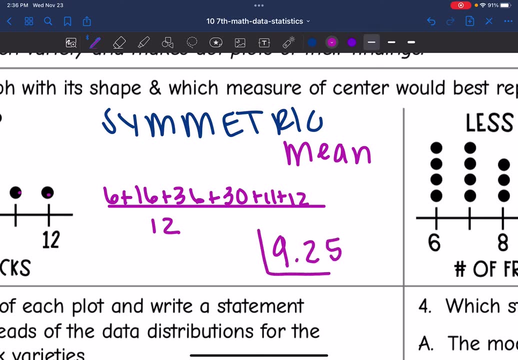 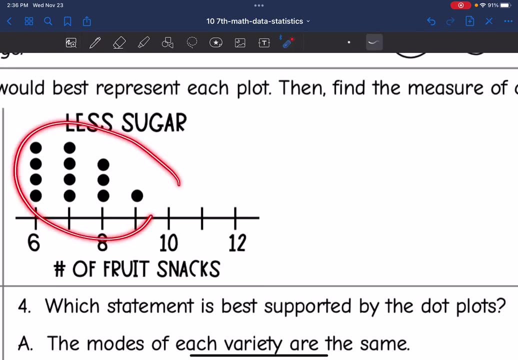 plus 30 plus 11 plus 12 is 111, and then 111 divided by 12 is 9.25.. So the mean is 9.25.. Okay, then the less sugar. this is pretty skewed to the right, since I have most of the data on. 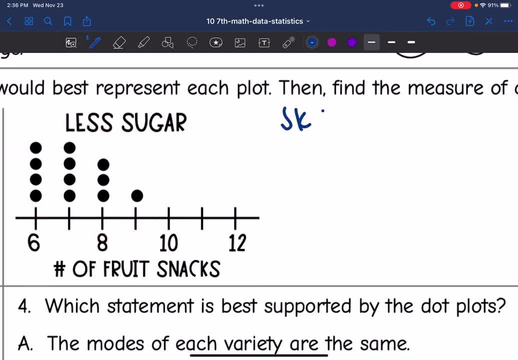 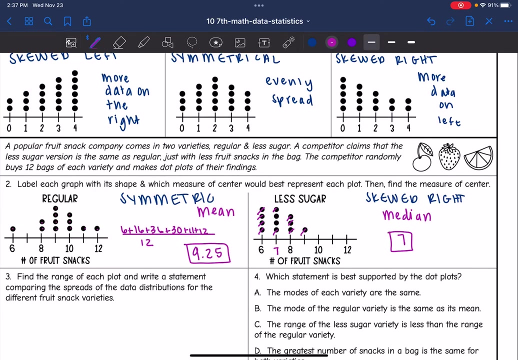 the left, So this is skewed right. and when I have skewed data, remember the median is the best center. So I'm going to go through and find the median of this data by finding the middle, and the median is going to be 7.. Okay, now let's answer some other questions. So number three says: find the range of each plot. 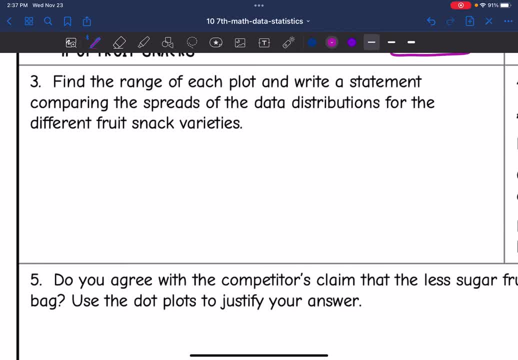 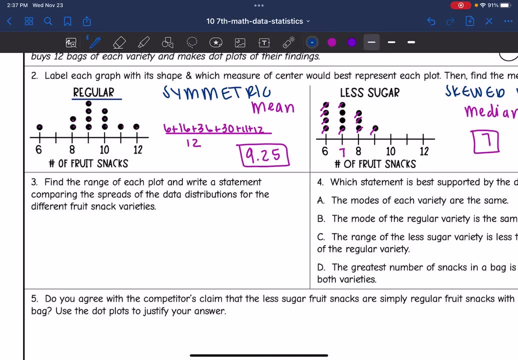 and write a statement comparing the spreads of the data distributions for the different fruit snack varieties. So let's start with the regular. Let's find their range. The highest range is 7.5.. So let's start with the highest range. The highest range is 7.5.. So let's start with the highest range. So let's start with the highest range. 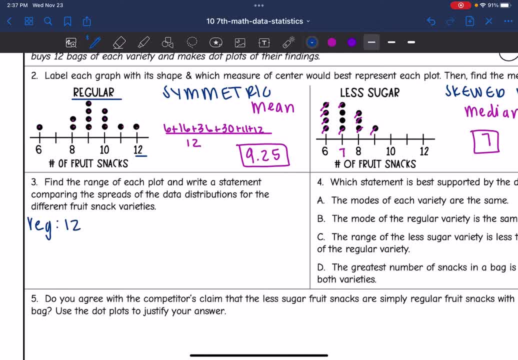 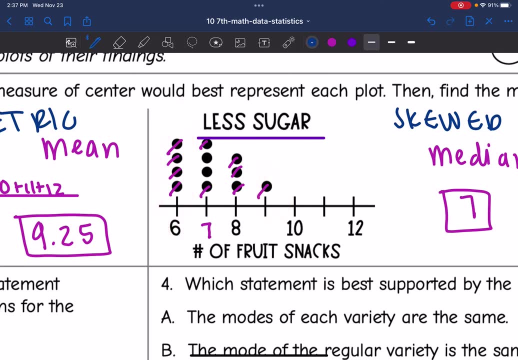 The highest number of fruit snacks in the bag was 12 and the lowest number was 6.. So 12 minus 6 is 6.. Okay, now let's look at the less sugar. Their highest was 9 and the lowest was 6.. So to find the range for the less sugar, 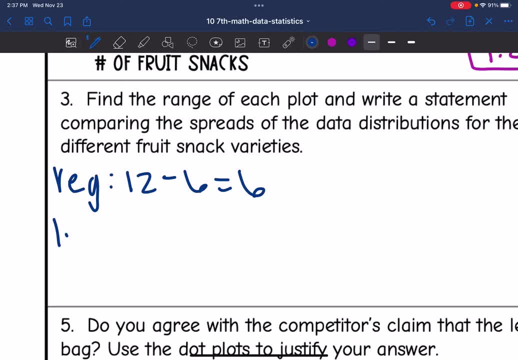 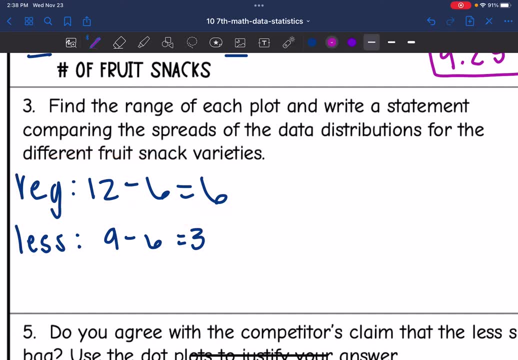 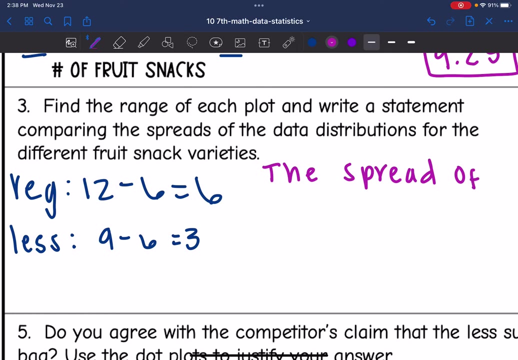 I would do 9 minus 6, which is 3.. So that means that the spread of the regular fruit snacks is larger than the spread of the less fruit snacks. The spread of the regular fruit snacks is larger than the less sugar fruit snacks. 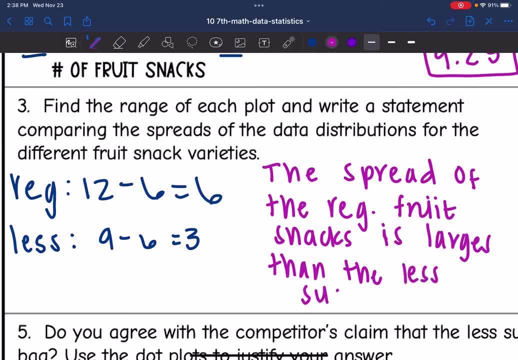 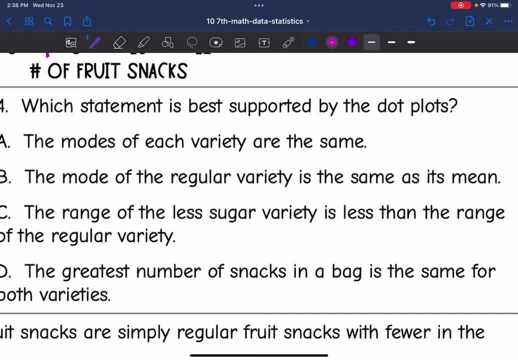 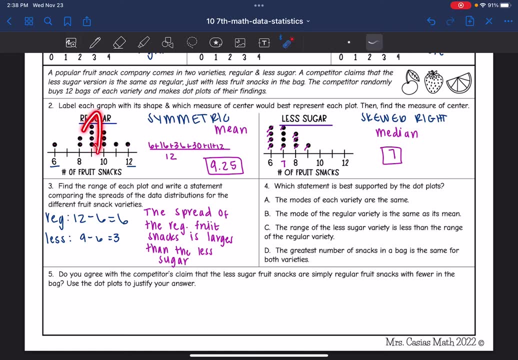 So to find the range, I would do 9 minus 6, which is 2.. 4 times 2 times 2 times 3 times 3 times 3 times 2 times 3 times 4 times 5 is not true. B says the mode of the regular variety is the same as its mean. So we found: 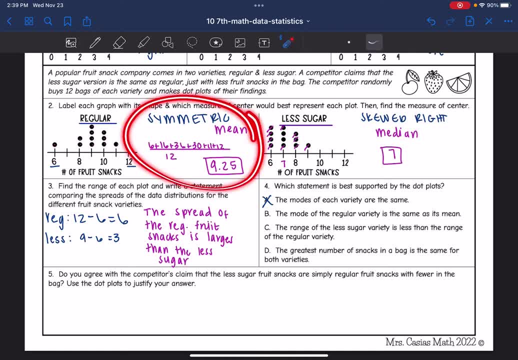 the mean of the regular variety it was 9.25, and the mode like we just talked about is 7.. So that's not true either. C says the range of the less sugar variety, which was 3, is less than the range of the regular variety, which was 6.. So that one is true. Let's read through D just to verify that. 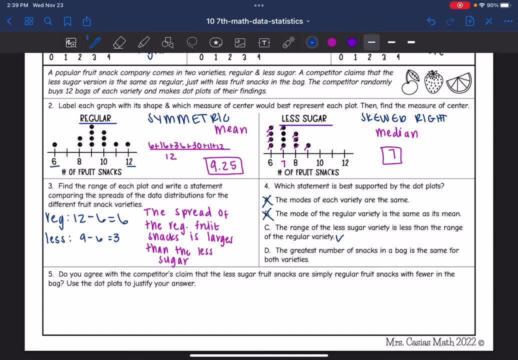 C is the correct answer. D says the greatest number of snacks in the bag is the same for both varieties. The greatest number of snacks in the bag is the same for both varieties. That is false because the less sugar the greatest number of snacks in the bag was 9, and the regular the 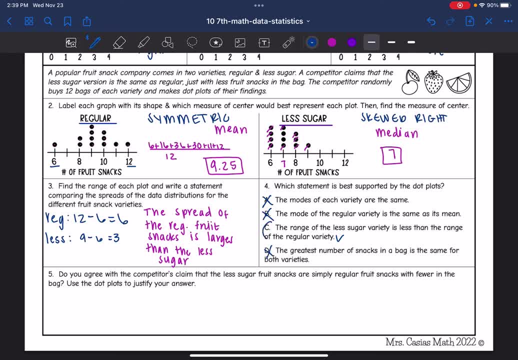 greatest number of snacks in the bag was 12.. So C is the correct answer there. And then five says: do you agree with the competitor's claim that the less sugar fruit snacks are simply regular fruit snacks? with it fewer in the bag, Use the dot plots to justify your answer. So I would say: